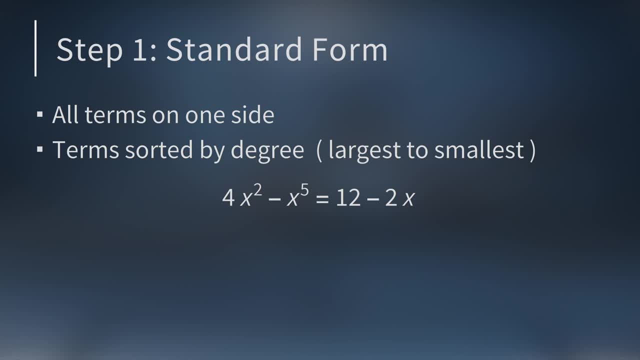 4x squared minus x to the fifth equals 12 minus 2x. If you subtract 12 from both sides, you get 4x squared minus x to the fifth. minus 12 equals negative 2x. Next add 2x to both sides to get. 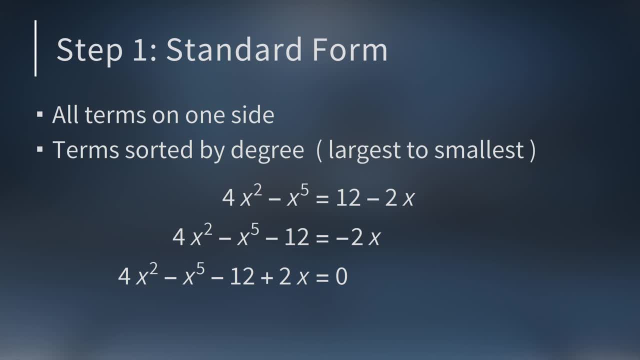 4x squared minus x to the fifth, minus 12 plus 2x, equals 0.. Now all the terms are on one side. This is a polynomial with integer coefficients, but it's not in standard form. Remember you write polynomials from largest degree to smallest degree. Once we do this, the largest exponent is 5,. 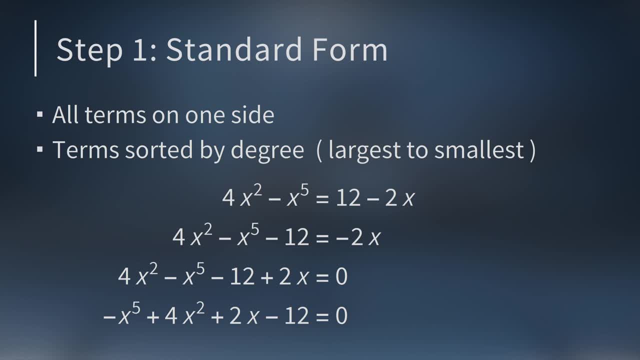 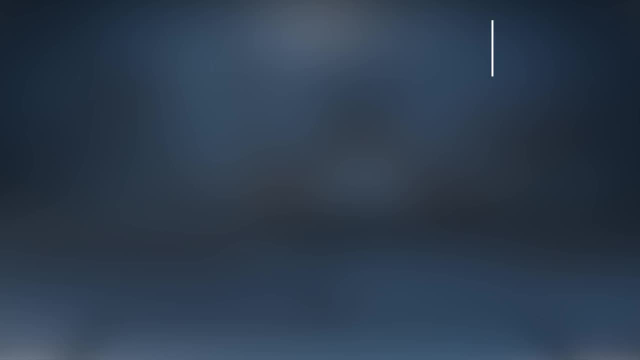 then 2,, then 1,, which you don't write, and then the constant term negative 12, which has degree 0.. Once our equation is in standard form, we'll check to see if 0 is the solution to the equation. 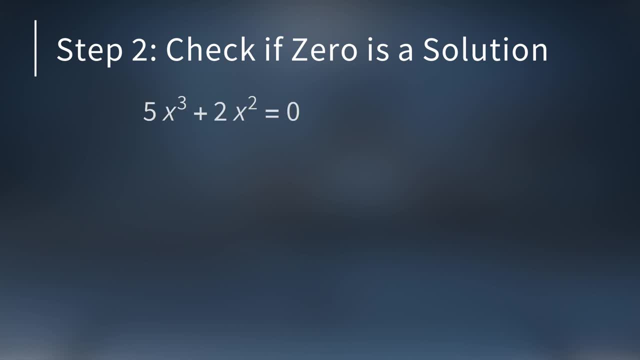 For example, look at the equation: 5x cubed plus 2x squared equals 0.. On the left hand side we can factor out x squared. This gives us x squared times. the quantity of 5x plus 2 equals 0.. 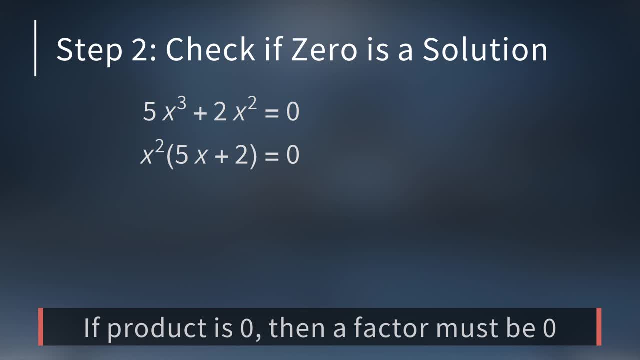 And a key principle in solving equations is that if a product of factors is 0,, then we're going to have a product of factors of 0. If a product of factors is 0,, then we're going to have a product of factors of 0.. 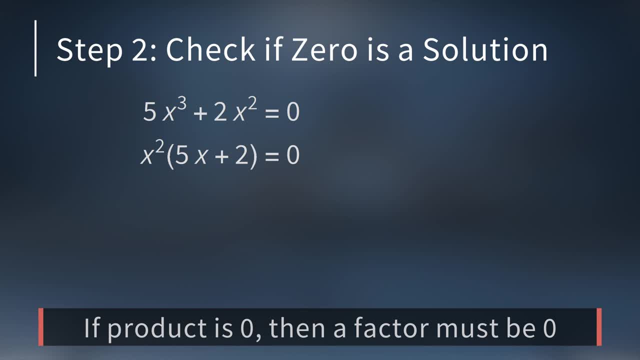 Then one of the factors has to be 0. This is because if you multiply a bunch of numbers together, the only way their product is 0 is if one of the numbers is 0. Once we do this, we see the solutions are 0 and negative 2 fifths. So this Diophantine. 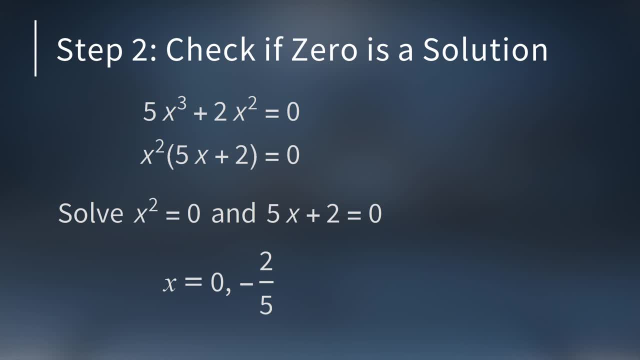 equation does have an integer solution: 0.. Quick note: when solving a Diophantine equation, sometimes you'll want to find all fraction solutions and not just the integer solutions. In that case, you'll want to find all fractions solutions and not just the integer solutions. In that case, you'll want to find all fraction solutions and not just the integer solutions. 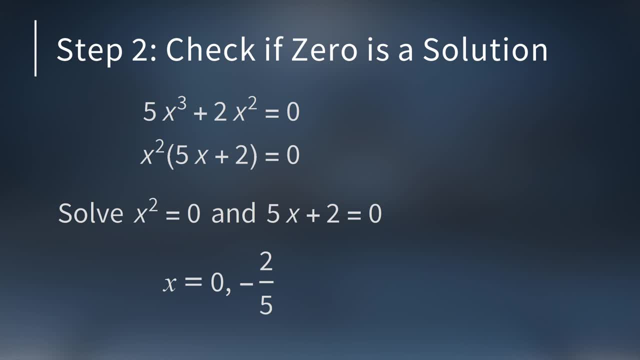 case, we did just find all the rational solutions- 0 and negative 2 fifths, but today we're focused on finding the whole number solutions. For another example, look at the Diophantine equation: 3y to the 7th minus 4y squared plus. 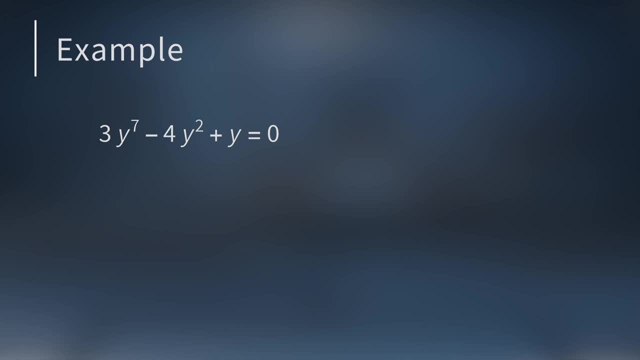 y equals 0.. All the terms are on one side and the polynomial is in standard form, so the first step is done. We can factor out y, which gives us y times the quantity of 3y to the 6th, minus 4y plus 1 equals 0.. Setting the first factor to 0 gives us one integer. 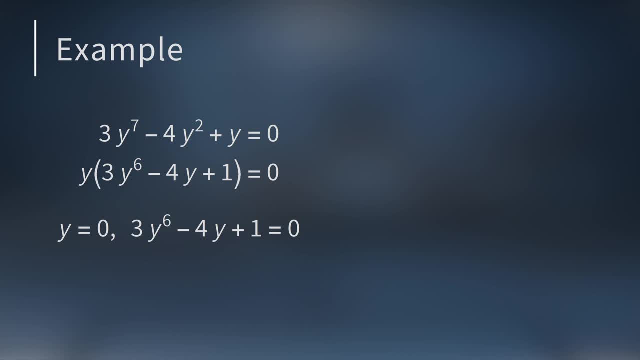 solution: y equals 0, but what about the second factor? Is there a straightforward way to tell if 3y to the 6th minus 4y plus 1 equals 0 has an integer solution? You could always graph it and see if it crosses the x-axis anywhere near an integer. The problem with 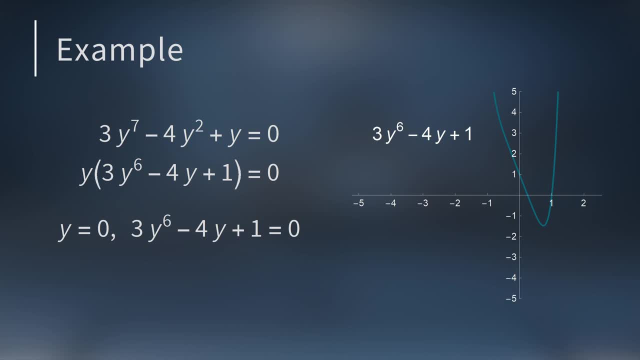 this approach is for very large polynomials. You have to do some work to see how large the graph needs to be to be sure you are seeing all of the x-axis crossings. Also, it involves eyeballing the graph. It would be much better. 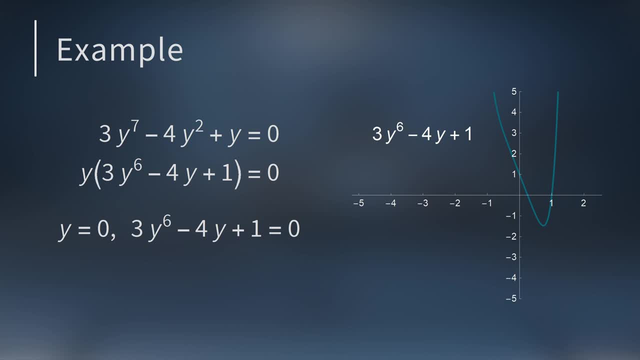 to have a simple, fast algorithm that would find all integer solutions. And it turns out that one such algorithm exists. You can write a program to quickly find any and all integer solutions. The key to finding the non-zero solutions lies in one simple trick. 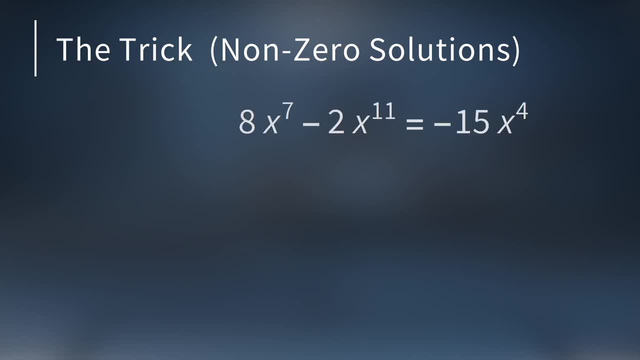 And the best way to see this is with an example. Let's find all integer solutions to the Diophantine equation. 8x to the 7th minus 2x to the 11th equals negative 15x to the 4th. 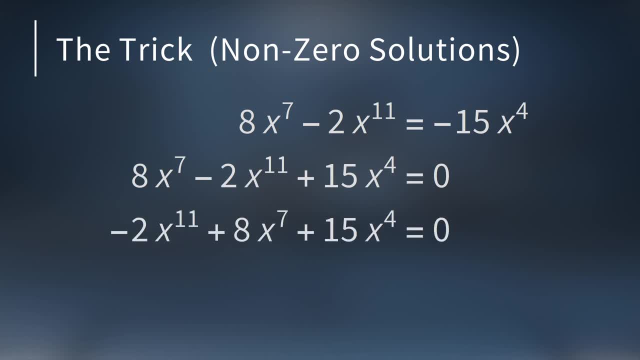 First get all terms on one side, Then rearrange them so the polynomial is in standard form. Next factor out the largest power of x For this equation, that's x to the 4th. So we know that x equals 0, is an integer solution. 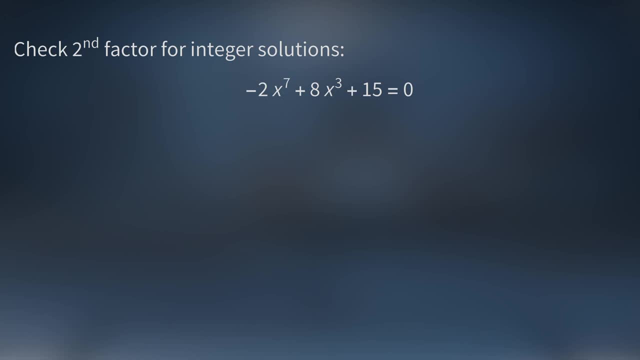 But now we have to check the second factor for any integer solutions. Here's the clever trick: Move the constant term to the other side. This means that every term on the left hand side contains a power of x. So let's simply factor out x. 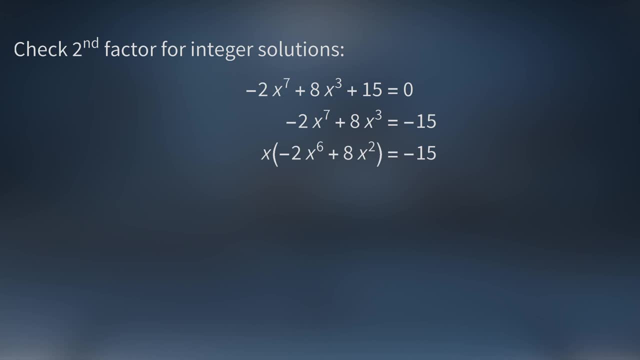 We could factor out x cubed, but to see the trick, we need to factor out just x. Our objective is to find any integer x that is equal to x to the 4th minus 2x to the 7th. That's the solution to this equation. 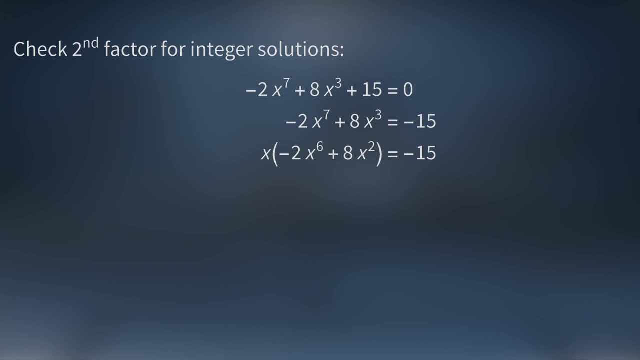 This means the first factor, x, needs to be an integer. But if x is an integer, then the second factor, negative 2x to the 6th plus 8x squared, will also be an integer. This is because all the coefficients are integers. 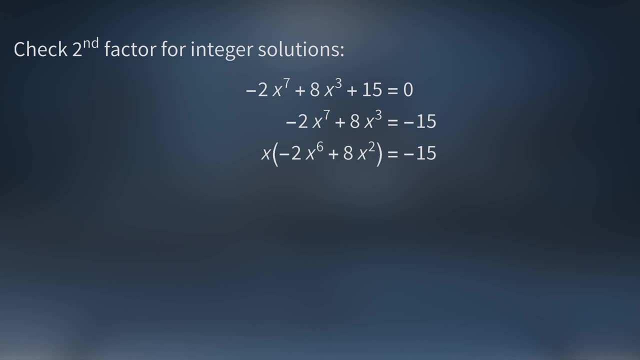 So on the left hand side, both factors are integers. This means that x must divide negative 15.. This is the key. All we have to do is make a list of all divisors of negative 15. And check them one by one. 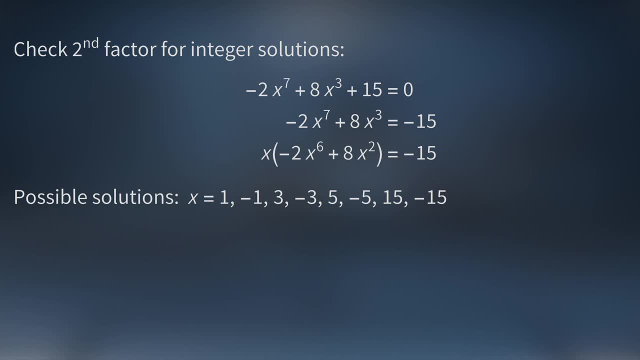 Here's a list of all possible solutions. They are all the positive and negative integers that divide negative 15. evenly, If we plug these numbers into the factor negative 2x to the 7th plus 8x, cubed plus 15, we get these eight values. 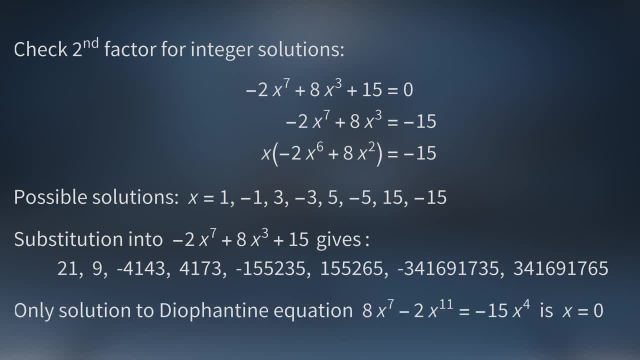 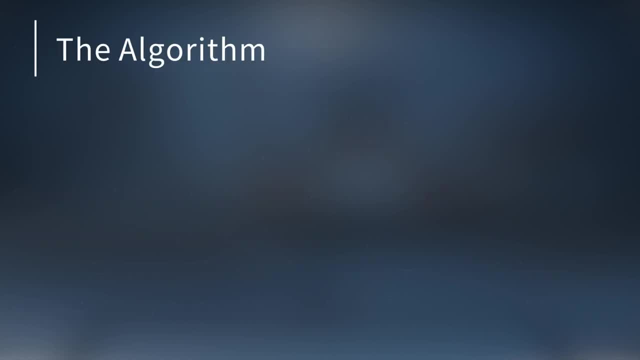 None of them are zero. so we're done. The only solution to the original Diophantine equation is: x equals zero. We're now ready to outline the algorithm to find all integer solutions to a Diophantine equation that's a polynomial with a single variable and integer coefficients. 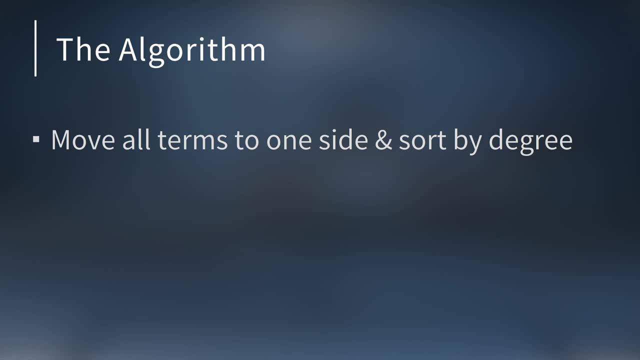 Step 1. Get every term on one side and sort them by degree. Step 2. Factor out the largest power of the variable. Step 3. Check all the divisors of the constant term in the remaining factor. You're done. 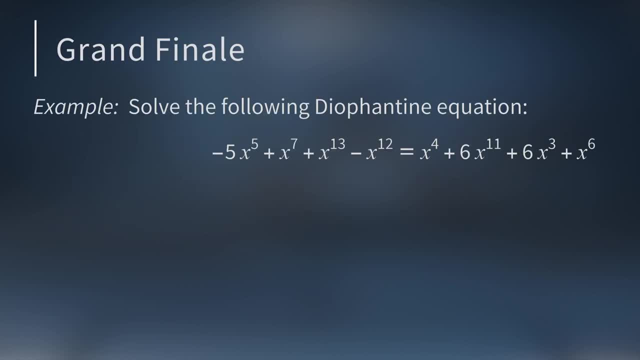 As a final example, let's solve this Diophantine equation. First, move all the terms to one side. Then sort this polynomial by degree, so it's in standard form. Next, factor out the largest power of x possible In this example, that's x cubed. 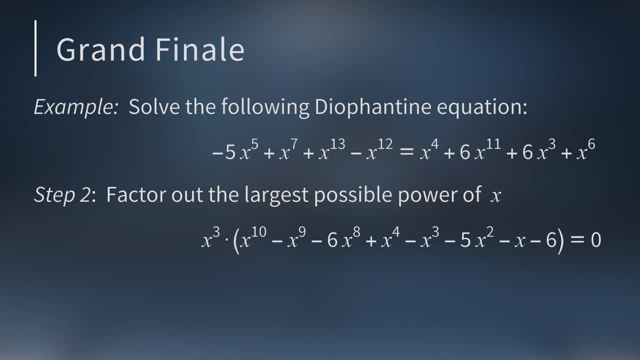 So x equals zero is a solution to this Diophantine equation. And now we want to check the polynomial in parentheses to see if it's ever zero. To do this, we check all the divisors of the constant term. The constant term is negative six. 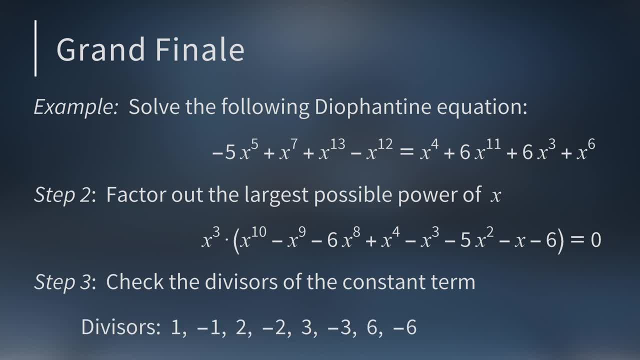 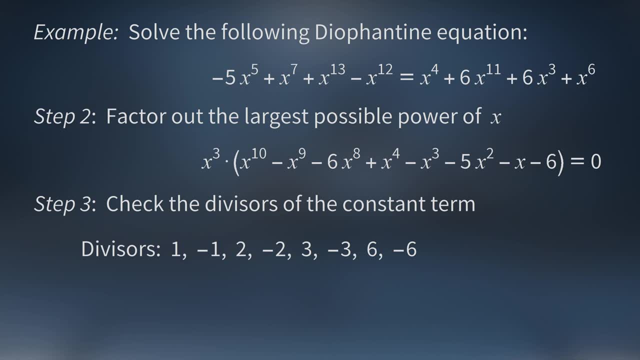 There are eight divisors: One negative one, Two negative two, Three negative three And six negative six. If you plug these eight numbers into the second factor, you get these eight values. The second factor is zero when x equals negative two or x equals three.